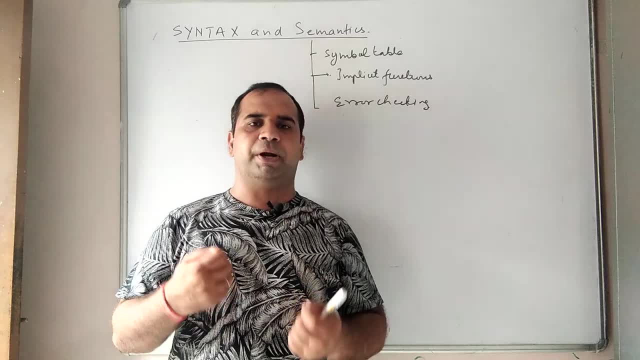 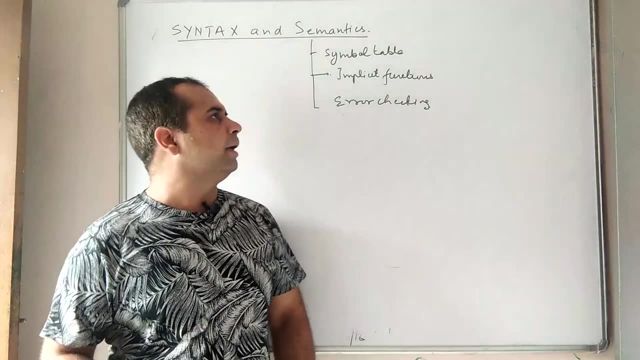 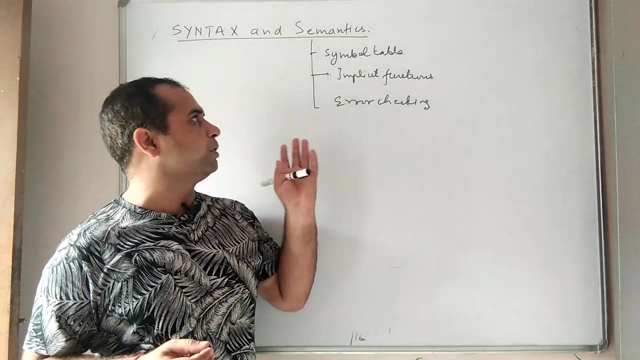 Look, the question of what is binding, what is binding time, what are different type of bindings, are frequently asked in principle of programming language subject. And another thing which is normally asked is that what is the difference between syntax and semantics? So today, at this moment of time, we will going to discuss syntax and semantics in a very short 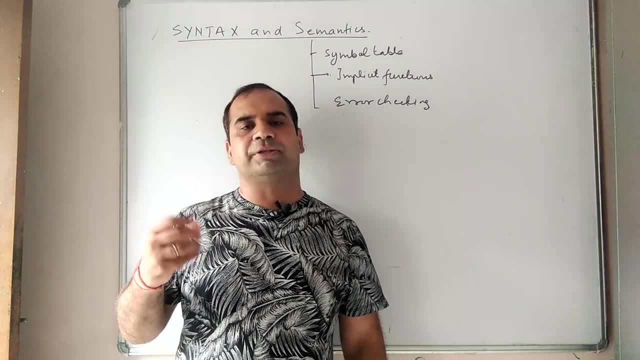 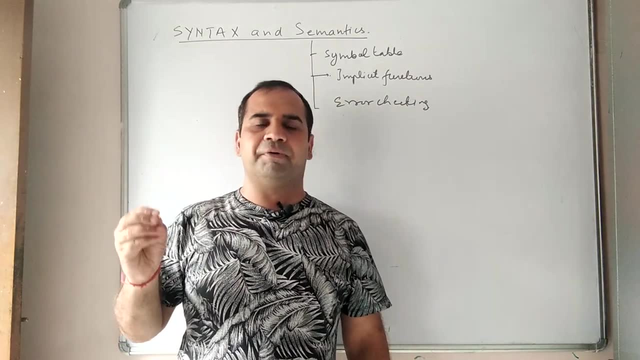 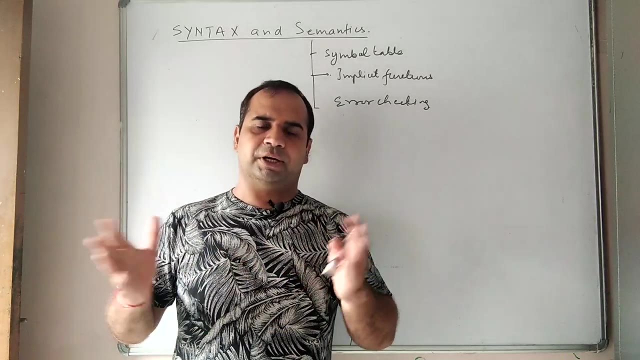 But the moment we will study the concept of translation, that is, compilation. there we will have steps of these phases And then- there I will dedicate a whole lecture on this- syntactic analysis and then semantic analysis. So there we will study it in more detail and we will get more ourselves, more involved in that. 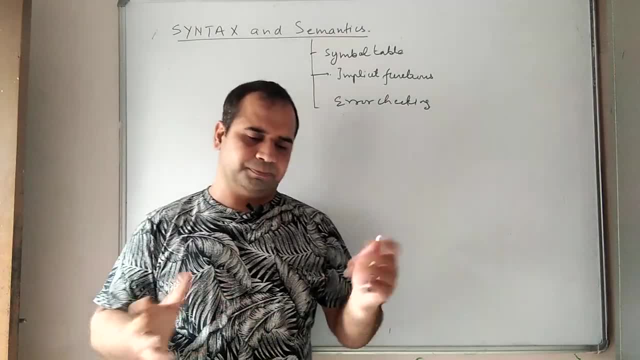 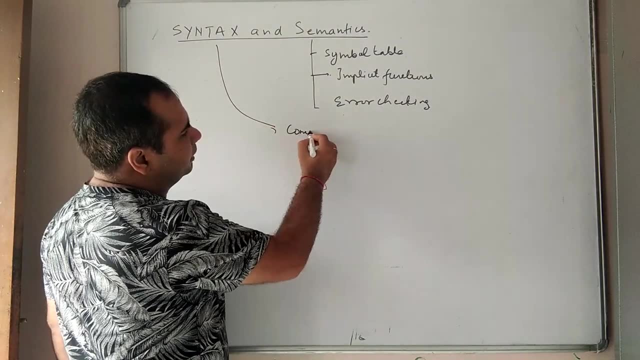 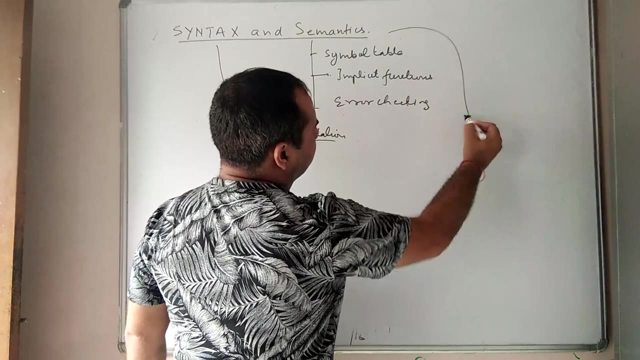 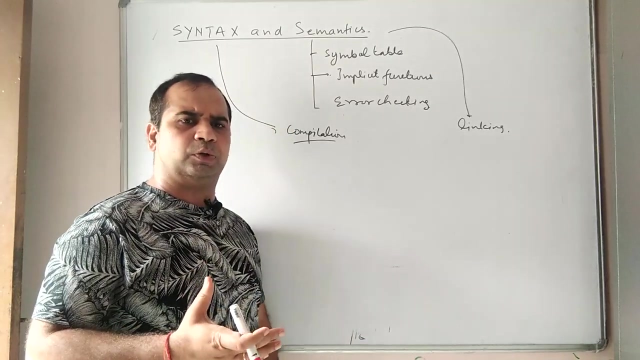 In that particular topic. So now start Syntax and semantics. Basically, the syntax syntax normally comes in compilation right And semantic semantic comes in linking phase right. So let us now try to differentiate between these so that when a question comes then you may be able to write in the difference form. 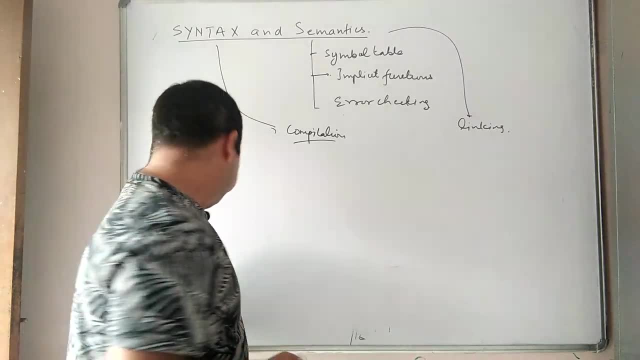 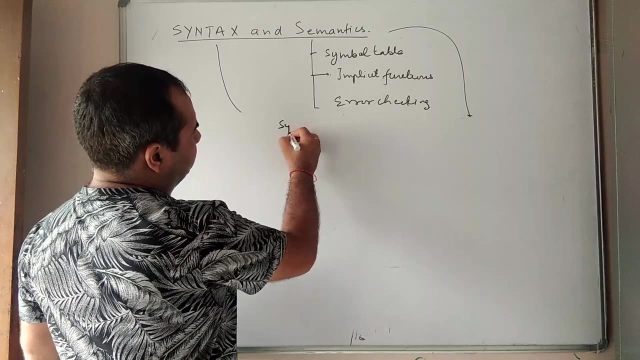 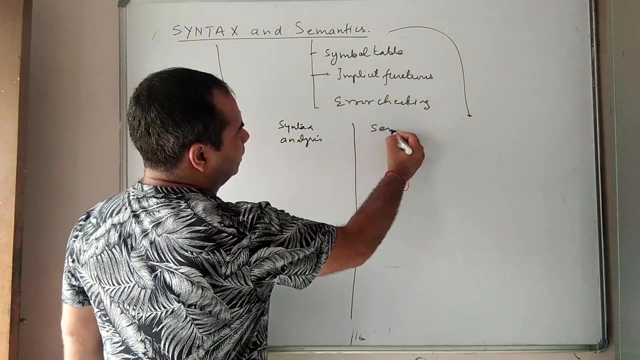 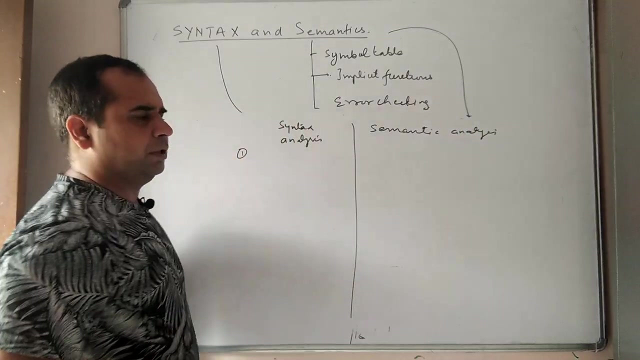 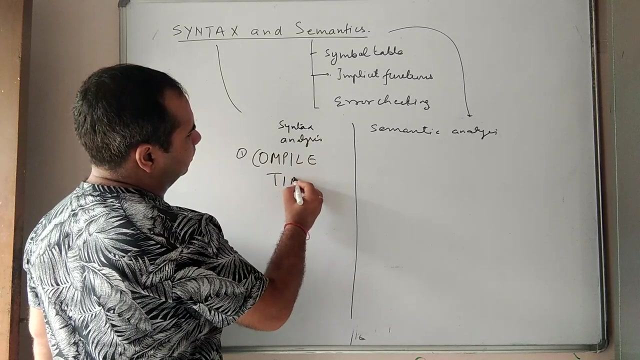 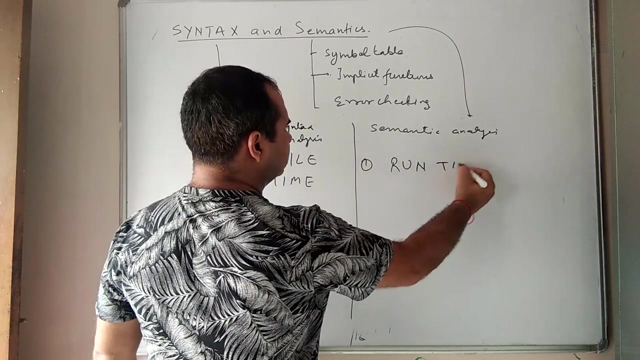 And so that it will be more clear to the examiner. So syntax analysis, and here we have semantic analysis. The first one is that the first important difference is that it is done at compile time, Whereas it is done at. we will go ahead in more detail. what is the difference between compile time and run time later on. 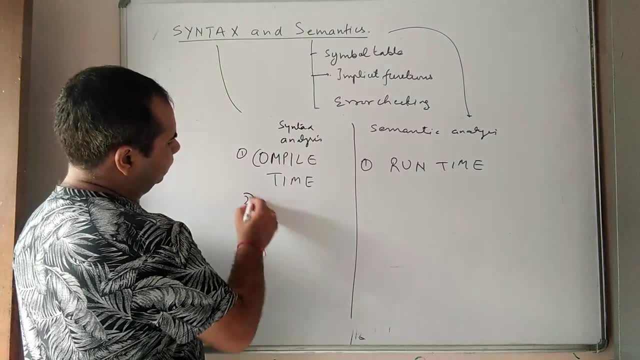 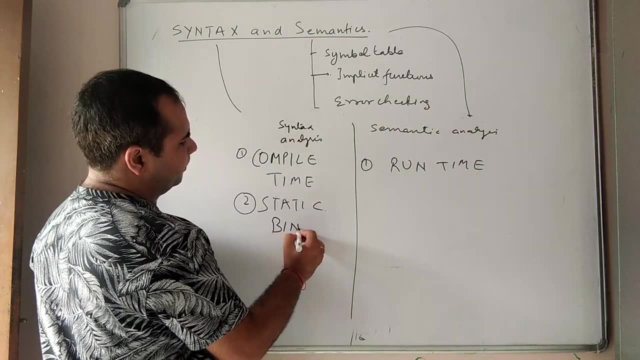 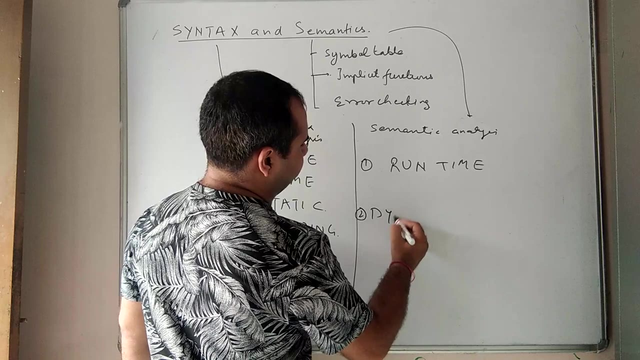 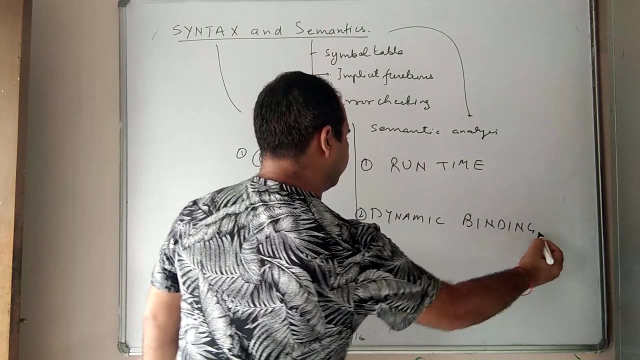 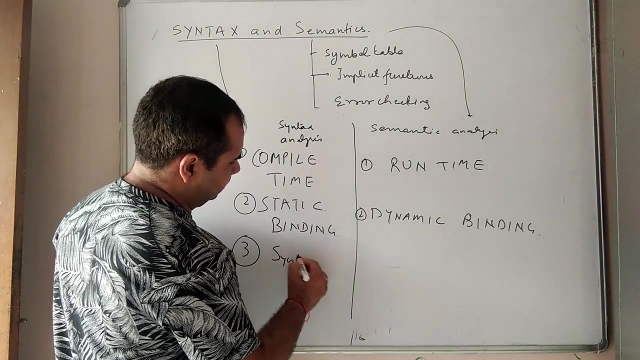 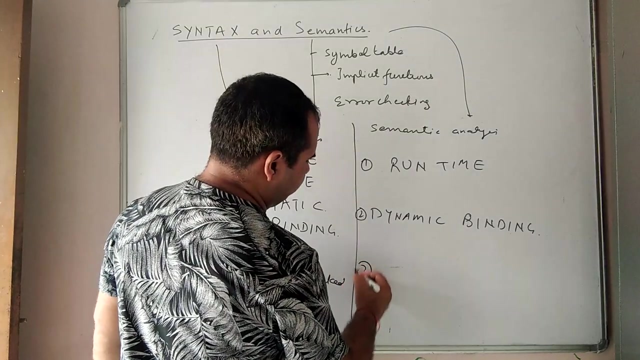 But at this moment of time, just to differentiate these two, we have to go for this. It is. it has static binding, B-I-N-D-I-N-G binding. It has dynamic binding. Number three: syntax get checked. Here we just check the syntaxes. 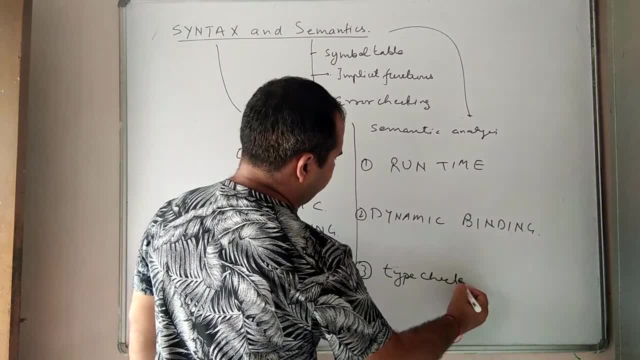 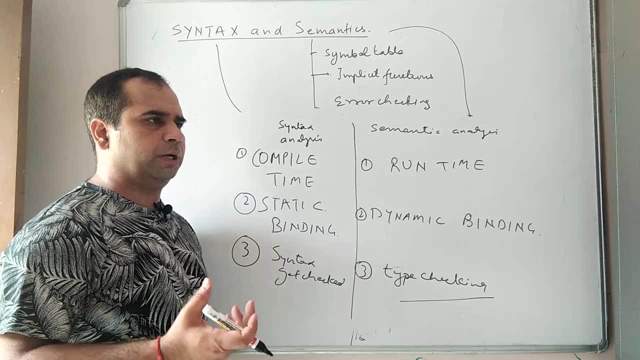 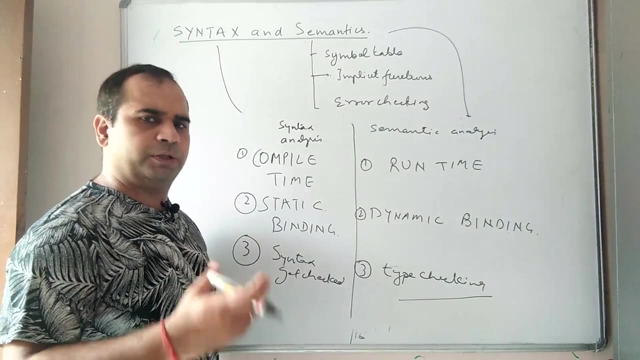 Type checking. Here we go, we move a step further and we check the type. So what is the type? It is the type of the variable, or is function is returning anything? If function is returning anything, it should not be void. and all these things. 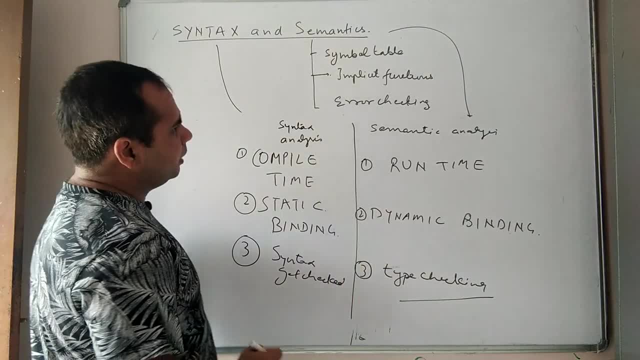 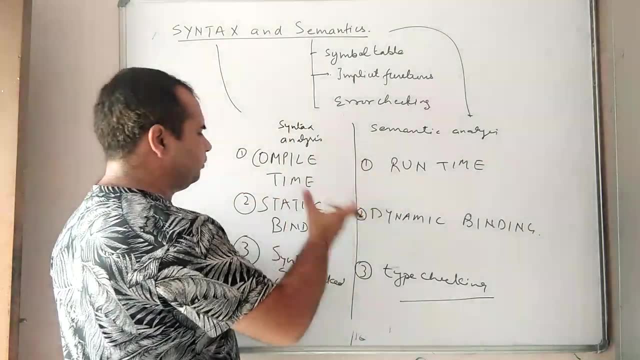 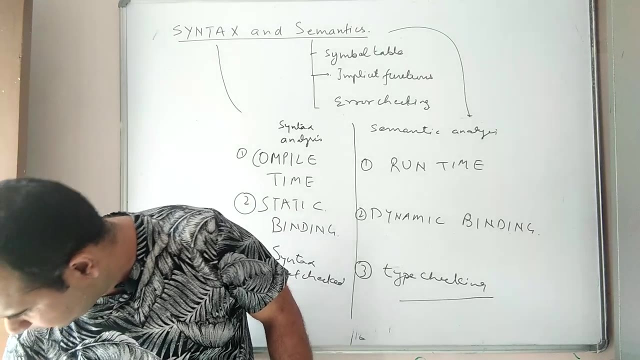 So these are the three important differences between the syntax analysis and semantic analysis And error checking is being done at compile time and run time. So these are the three broad differences. You can elaborate them and write good amount of answer to the in the question paper. 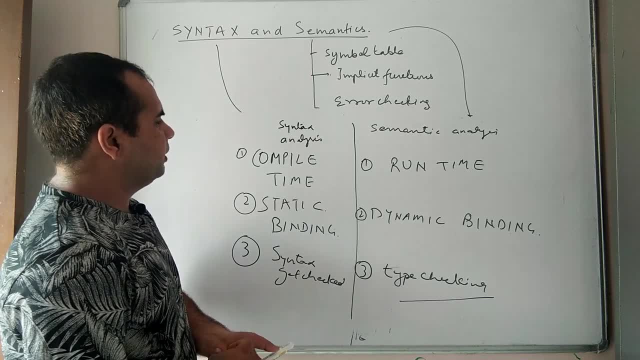 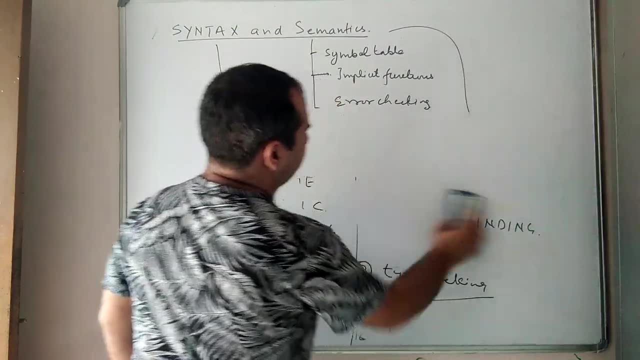 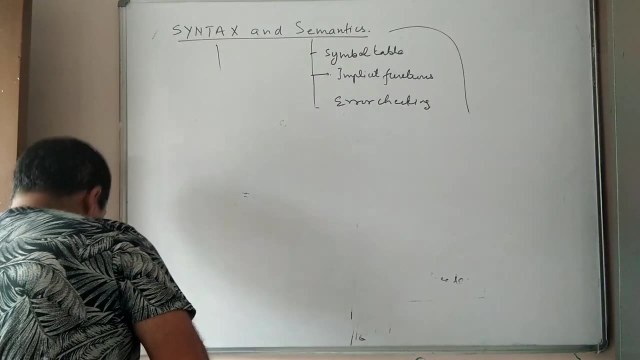 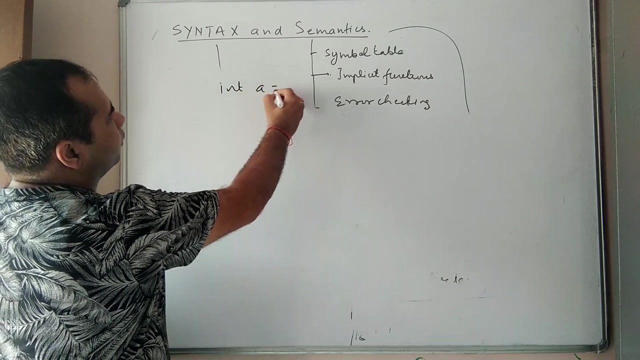 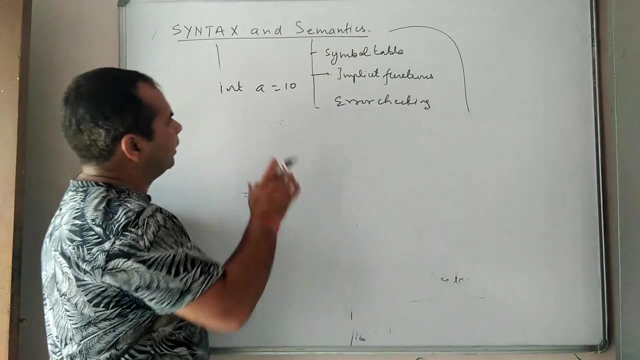 So let us now proceed step by step in syntax and semantic analysis with the help of an example. Suppose, if I will write integer A equal to 10- and I did not write any semicolon here- then this particular error will get through in compile time phase. 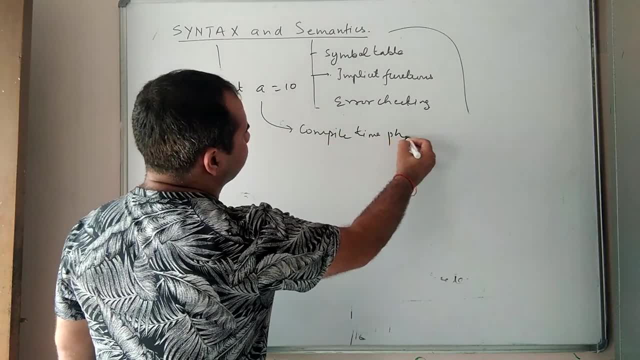 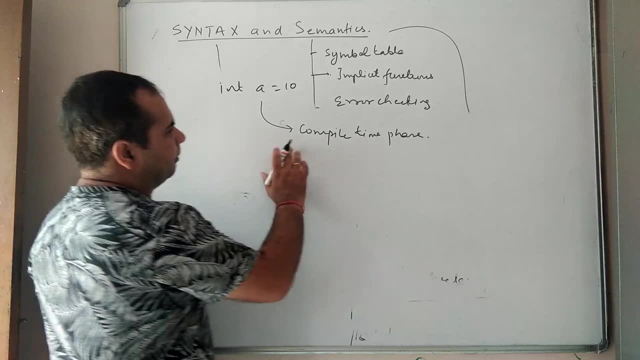 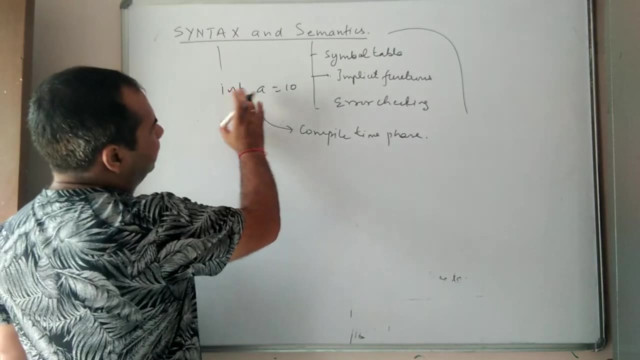 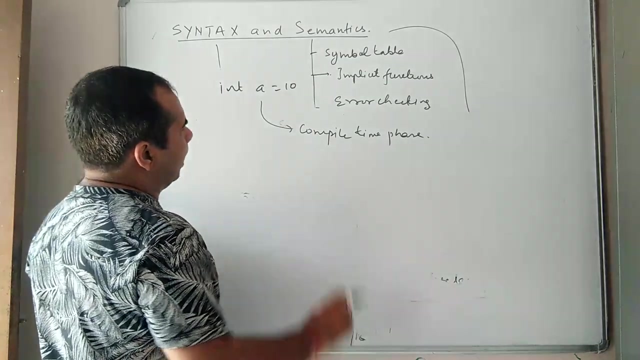 Compile time phase. Right, If I will write and compile time phase, because here the syntax is not correct. What is the syntax of C programming? The syntax is data type variable, and if you assign the value then equal to sign and the data 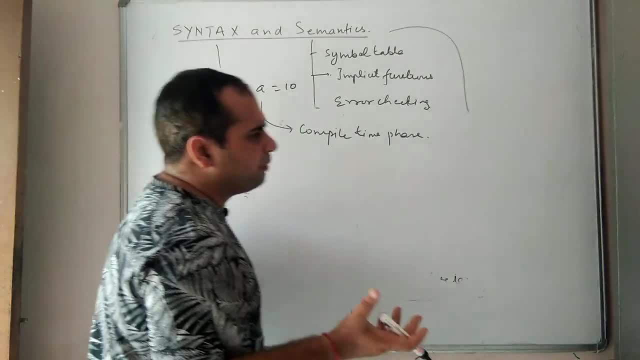 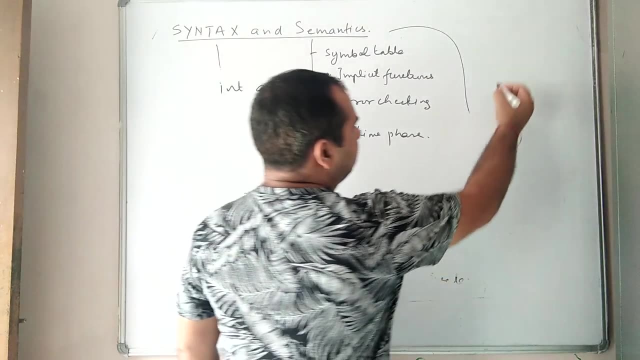 After then, to terminate the line, we have the semicolon. Then every language have its own programming constructs. But here we are talking about only C. If we talk about Python? in case of Python, we just need A equal to 10.. 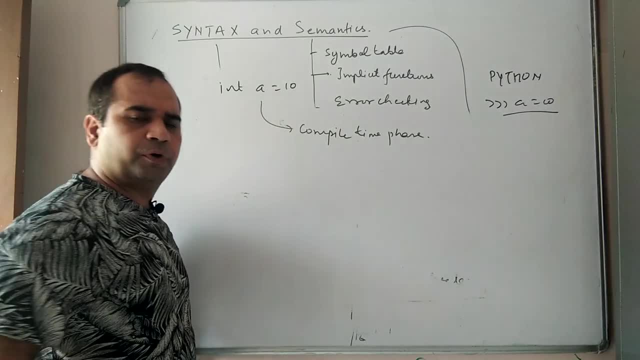 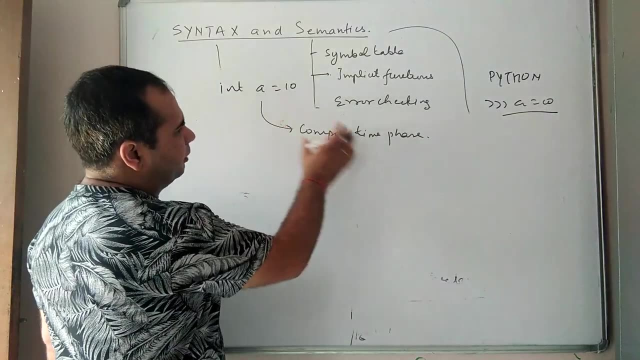 We do not need any type of data type declaration, because in it the whole concept is of dynamic binding. So compile time phase is there and this particular error will be checked in compile time phase. Now let us see an example where the error is being checked at run time. 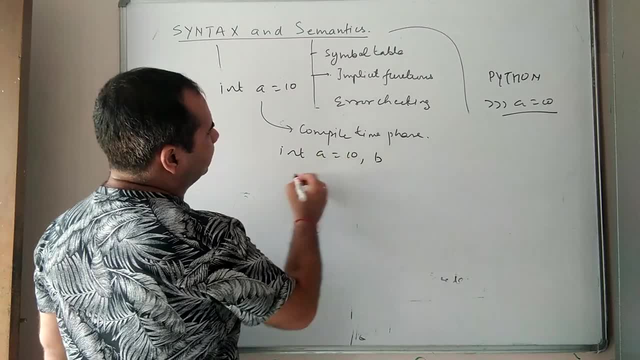 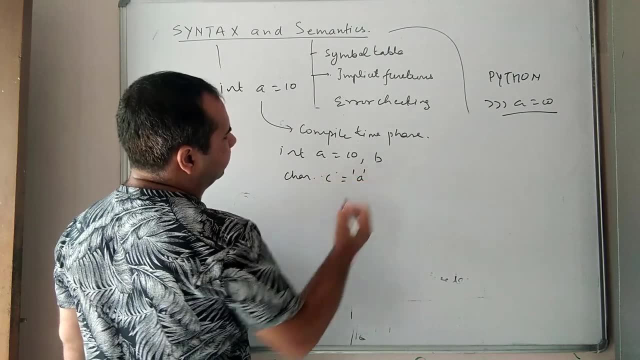 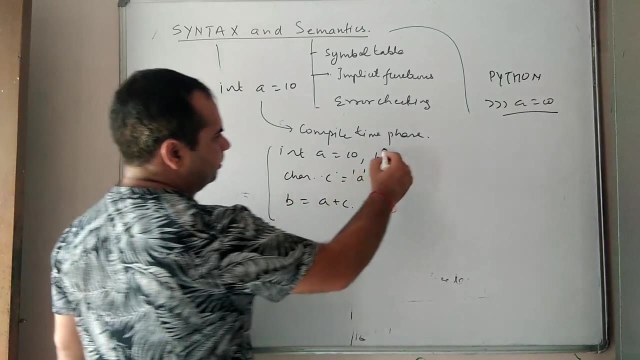 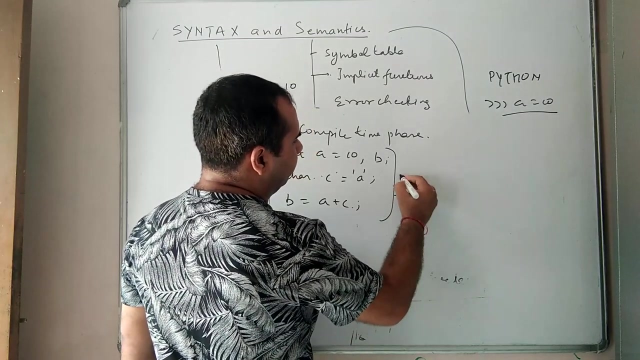 Integer A equal to 10 comma, B, char C equal to A and when we write B equal to A plus C. Now this particular phase. please see if I will write semicolon here properly. This particular phase will get passed easily without any error in compile time. 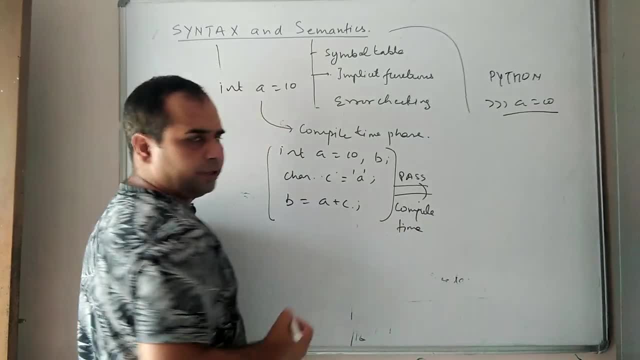 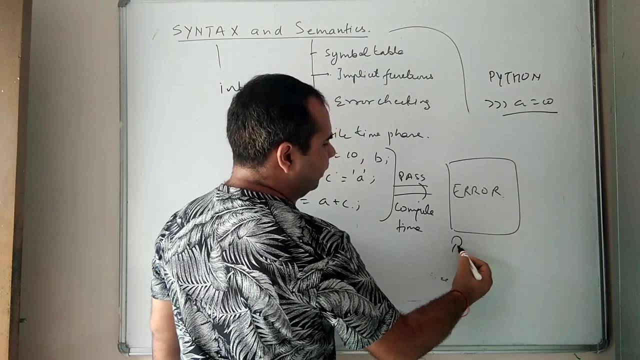 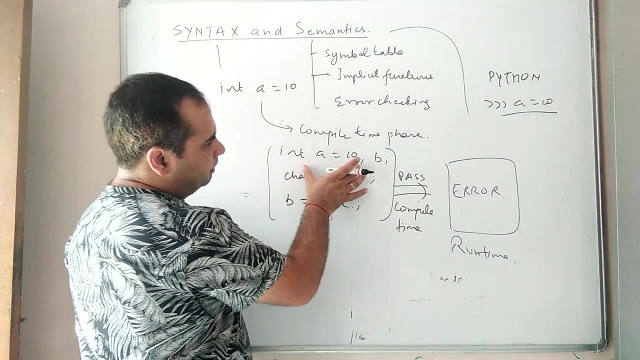 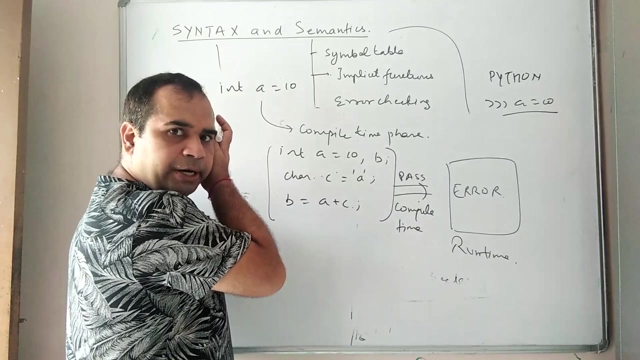 There will be no error in compile time. It is compilation time, But it will throw in error where In run time, Because syntactically this particular syntax is correct: Variable declaration is there, separator is there and terminator is there. Here also, all the stuffs are at the right place. 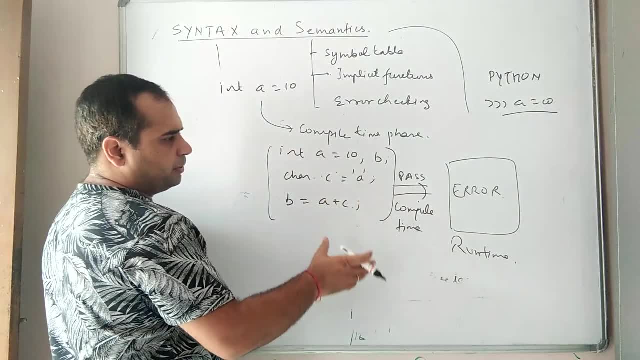 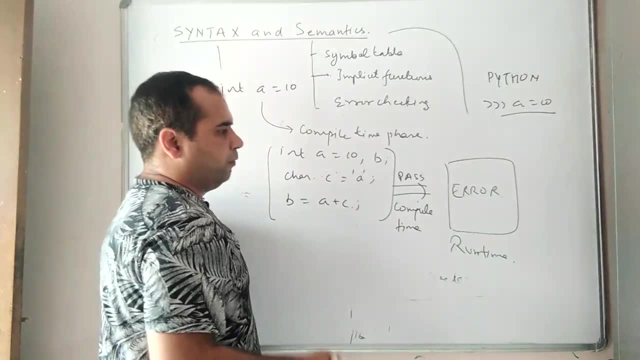 But when we come here in compile time it will get passed, but it get trapped in error In run time. Now, from where we get all these type of resources? From where this semantic analyzer control? all these things Will be from the symbol table. 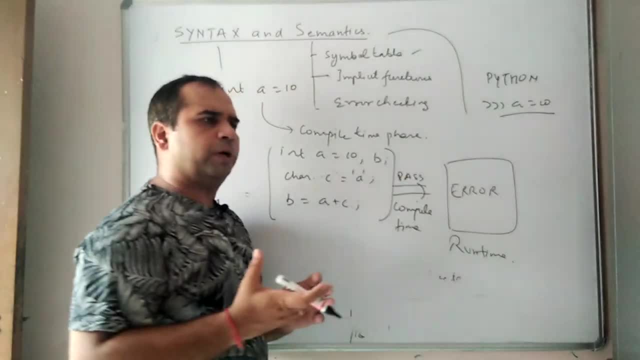 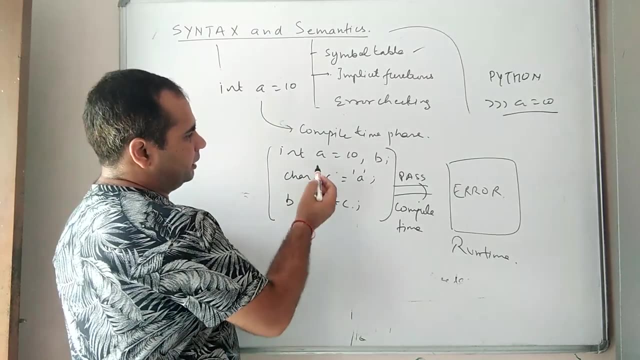 Symbol table is a collection of important elements and important definitions which play a very important role in type checking Means that if you are adding something, then it should be declared integer, or if you are using float, then it will produce the values in decimal. 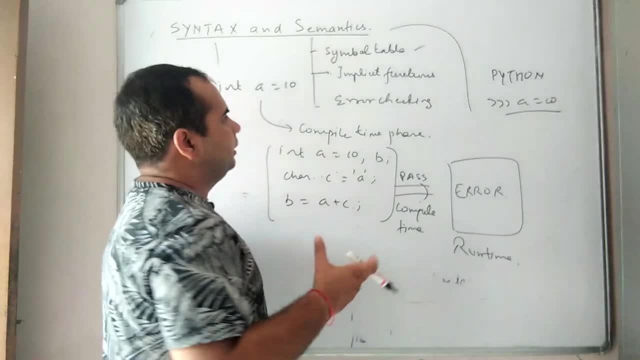 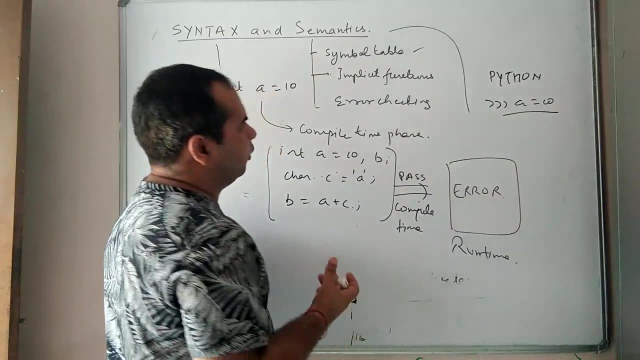 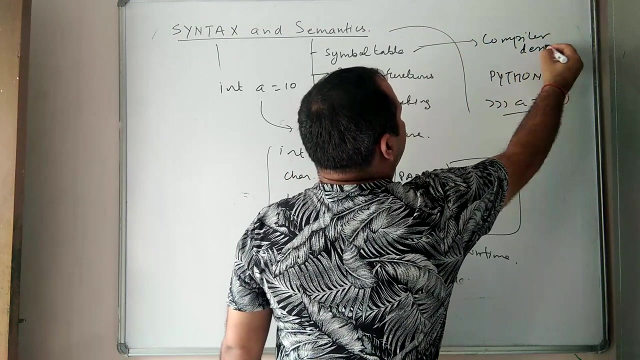 All these important stuffs are being stored in the symbol table. The definition of constant: if you have write constant, you can't change that particular value. So all these things are being stored in a symbol table. You will read more when you will study compiler designing. 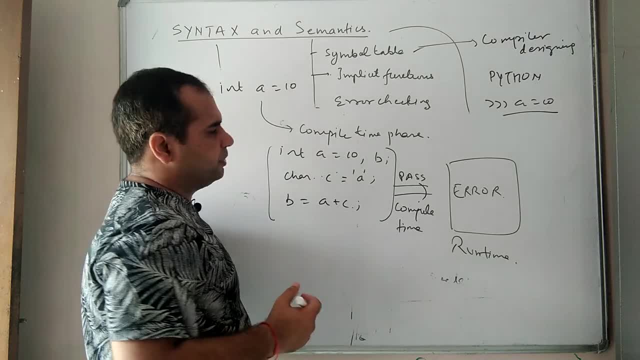 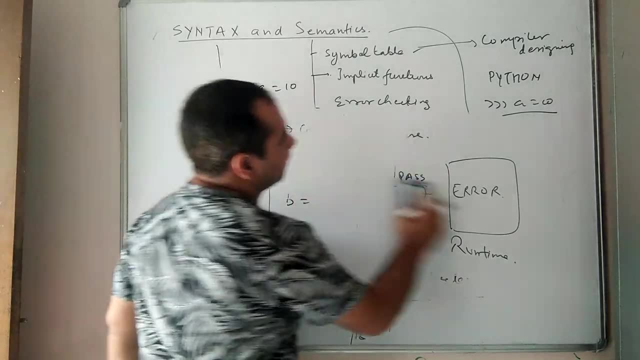 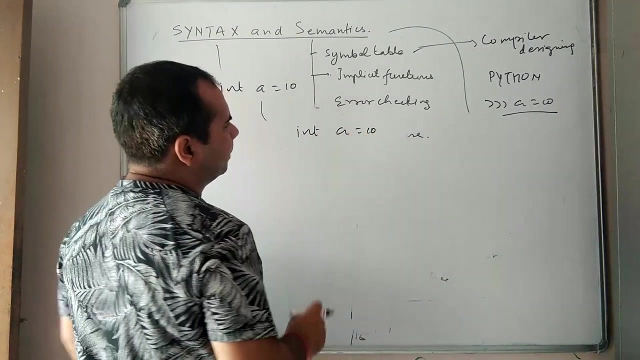 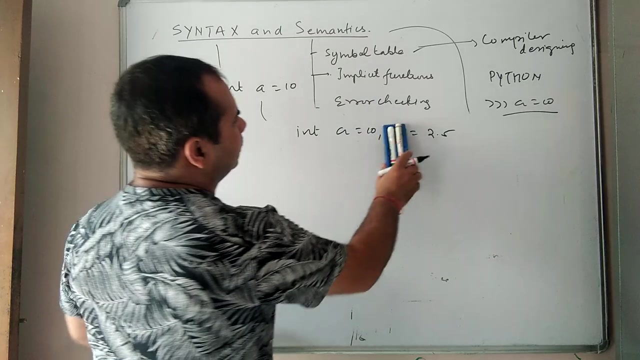 Now, next is implicit functions. Now, what is the rule of implicit function? is that suppose to explain the concept of implicit function? let us take an example. In the example integer a, equal to 10, is there And b, equal to 2.5, is there. 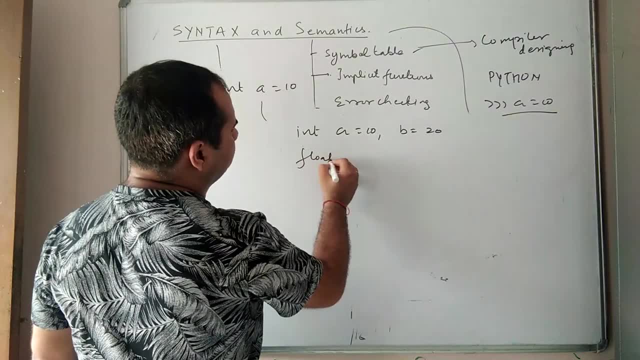 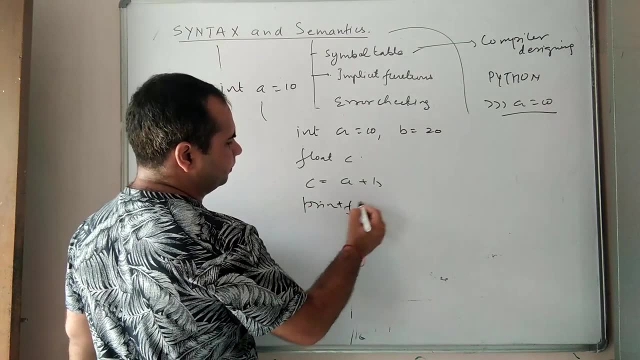 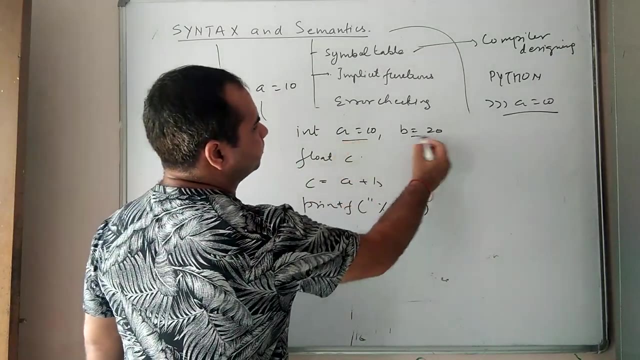 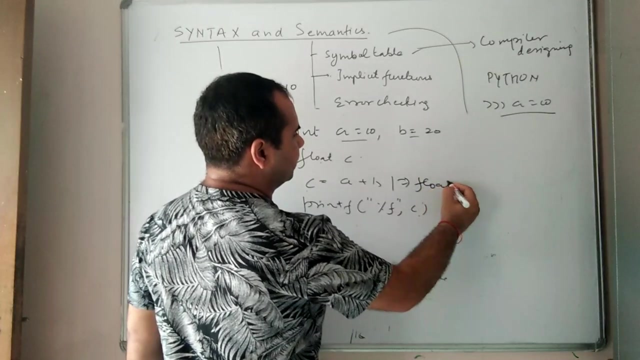 b equal to 20 is there And I have chosen float c, right, And I write c equal to a plus b When I write printf then since they both are integers and I have tried to produce the result in float, So implicitly what happens? that float a plus b occurs, right? 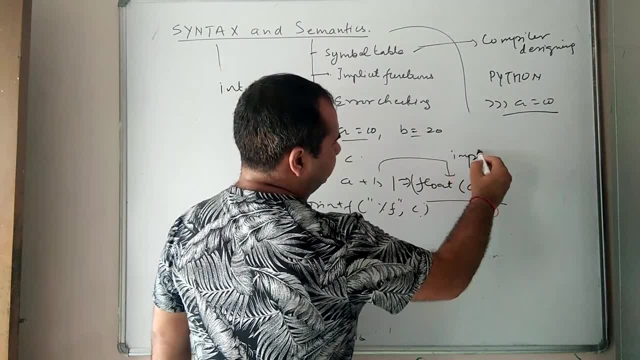 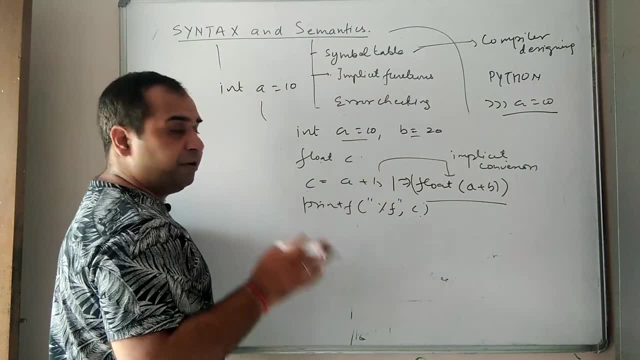 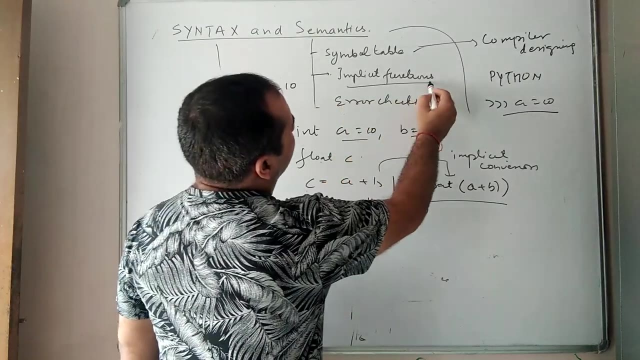 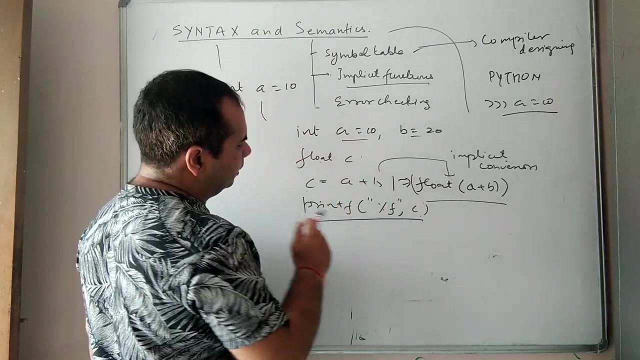 This is also known as implicit conversion. This I haven't written, But that happened in the background. This is known as implicit conversion. So implicit conversion will be done through the implicit function right And there, and after then we produce the output with the help of the percentage f and c. 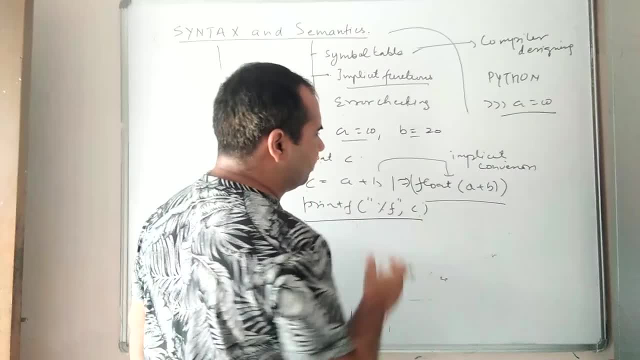 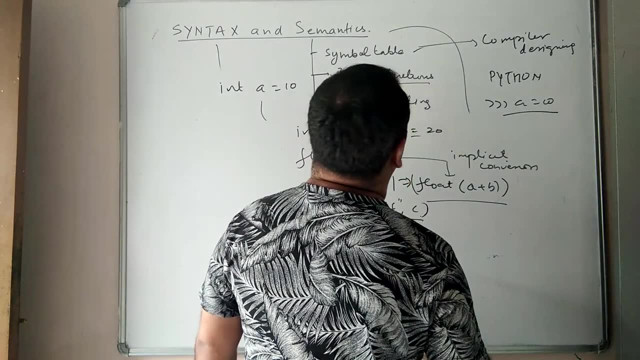 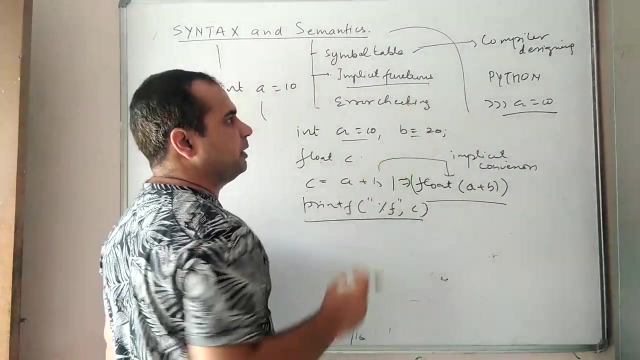 So implicit functions. this is just an example of symbol float function, But it can have a number of functions either, And after then there is error checking. So the error checking is of course going to be done depending upon the symbol table, the definition written in symbol table right. 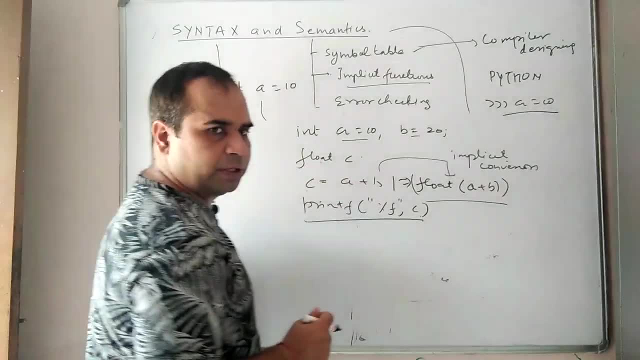 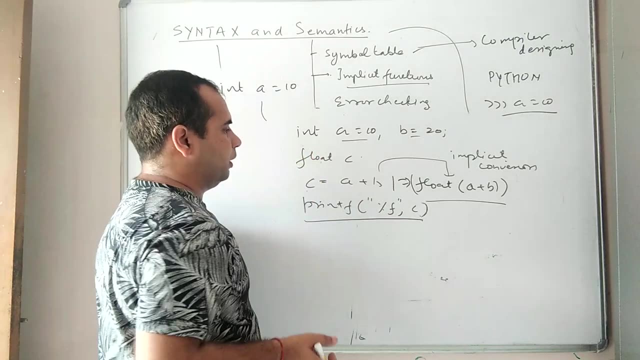 If it is, since float and integer are compatible with each other, only the way of representation is different. If there will be some other different data type, then maybe this particular data type conversion will not get acceptable And the error will be there. 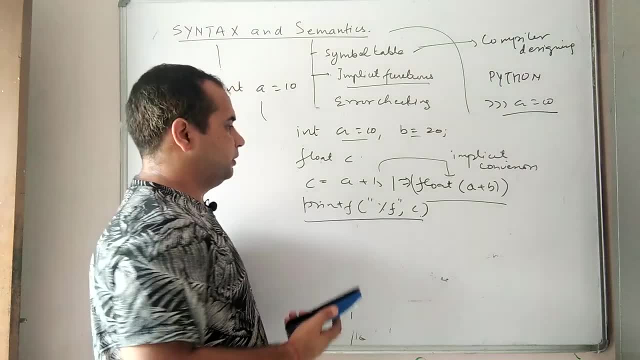 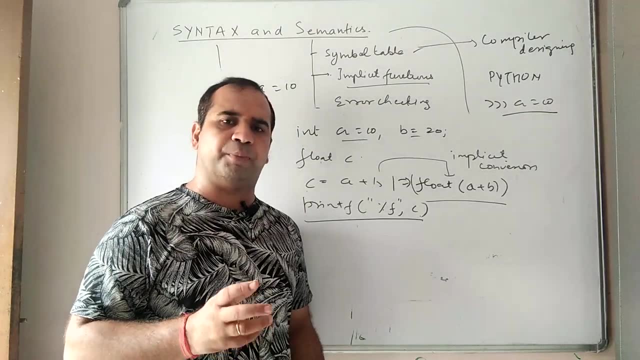 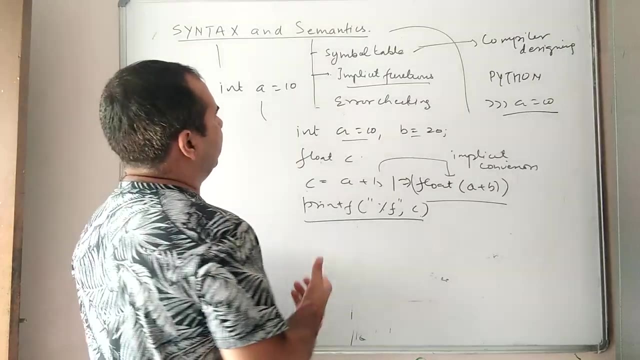 So all different type of error checking are being done here in the cementing analyzer. There are very important phases there. So all because before doing the data manipulation, before doing any type of operations, the whole soul of the computation of an expression is dependent upon the cementing analyzer. 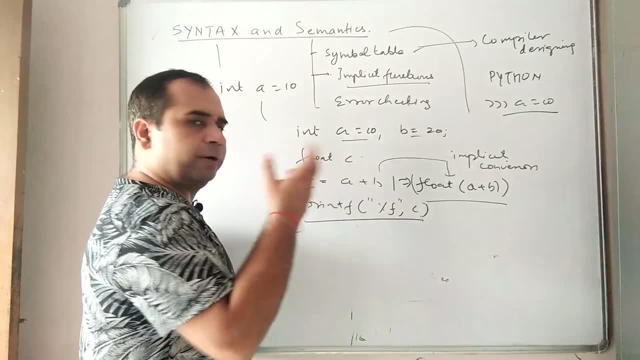 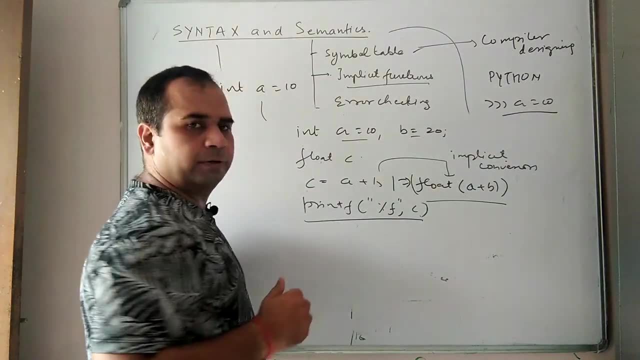 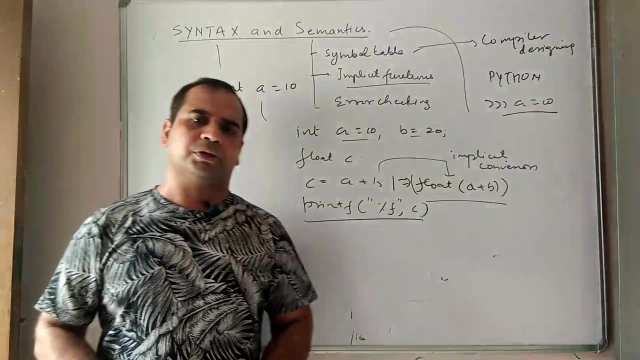 And the structure in the whole is dependent upon the, dependent upon the, this one synthetic analyzer right. So this is all about the syntax and semantics at this particular moment of time, And then we are going to discuss it further And in the next lecture we are going to discuss the binding time. Thank you very much.